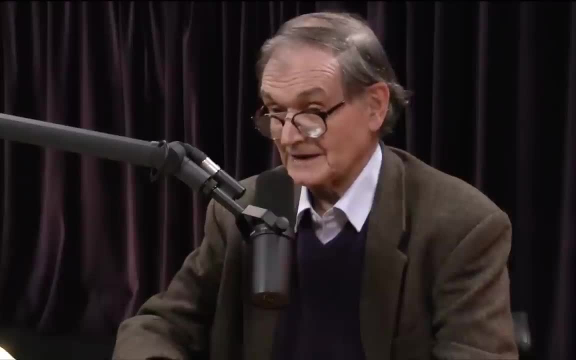 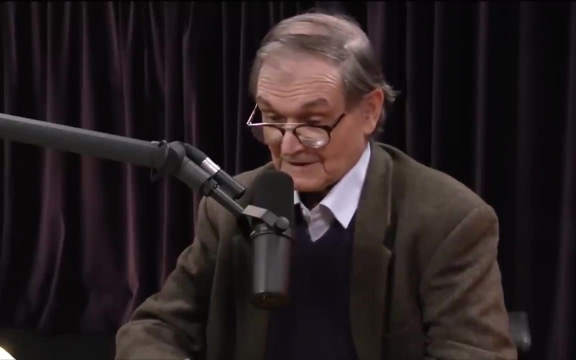 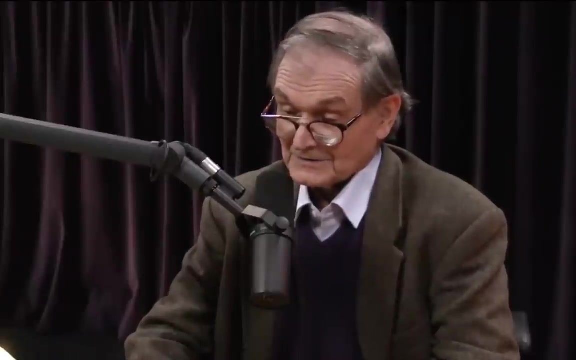 So these rules, you know they could be adding A and B, It's the same as B and A and things like that. And you say to the computer say here is a theorem like Goldbach conjecture And you see whether it can be proved. and you say maybe I've got a proof and this follows these steps. 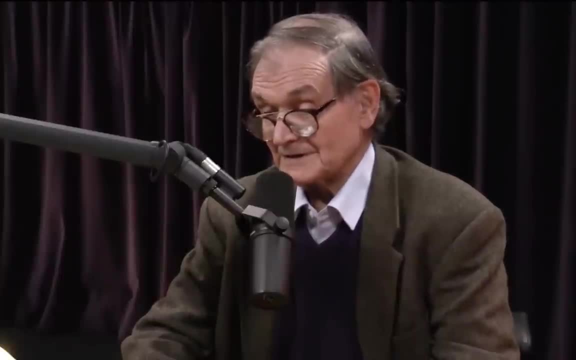 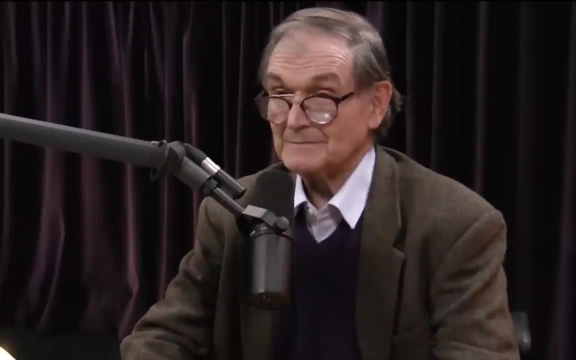 And you give it to the computer and it says, yup, you've done it right, it's true. Or maybe it would say, you've done it right and it's not true. Or it may not say anything, it might just go on forever. 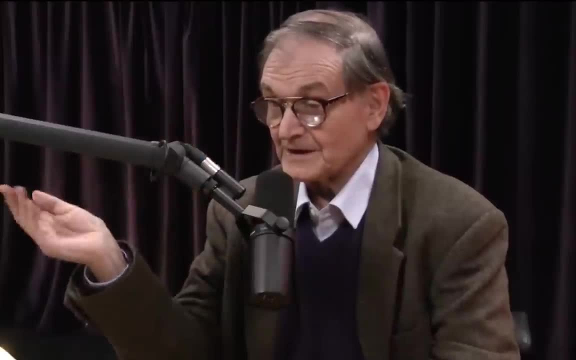 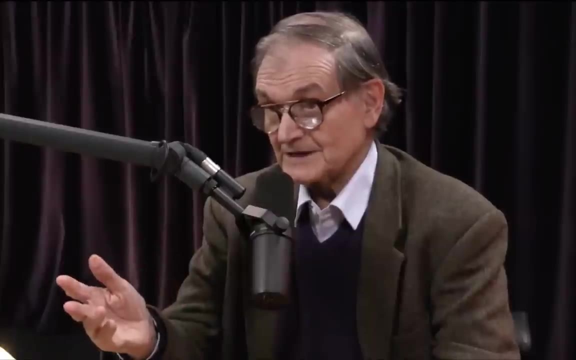 But these are the sort of outcomes, And the point about it is that if you believe that these procedures do give you a proof, in other words, that if the algorithm says yeah, it's true, then you believe that it is true. 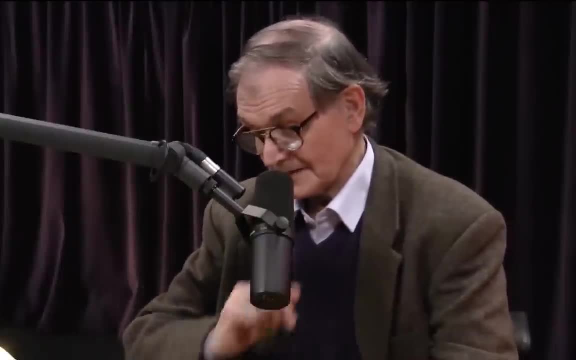 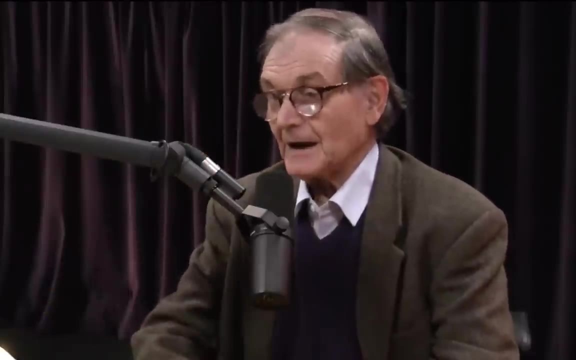 Because you've understood all the rules. You looked at the first one and said, yeah, That's okay. You looked at the second one and said, oh, yeah, I see. Okay, that's great, And you go all the way down. 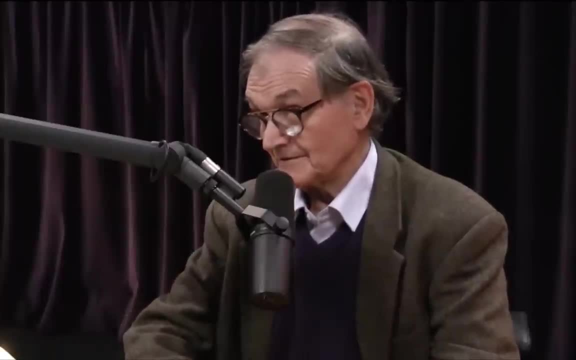 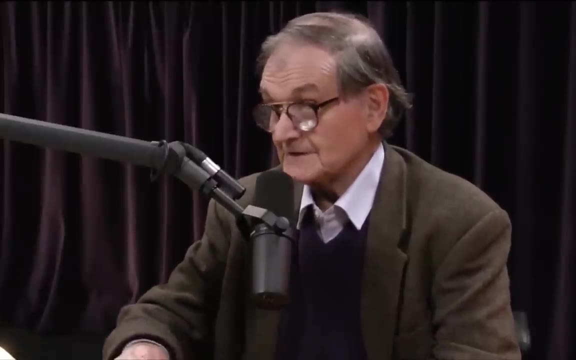 And as long as you're convinced all those rules work, then if it says yes, that's something you believe. Okay, Now what Gödel shows is he constructs a very specific sentence, a statement which is a number thing like the Fermat's Last Theorem or something, the thing about numbers. 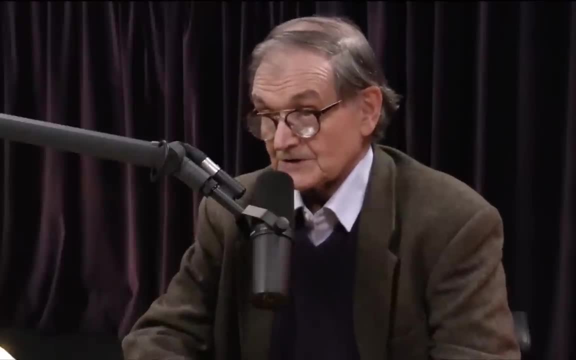 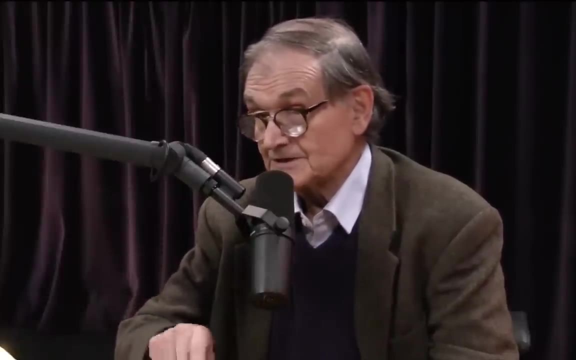 which what he shows is: if you trust this, this algorithm for proving mathematical things, then you can see, by the way it's constructed, that it's true, But you can also see, by the way it's constructed, that it cannot be proved by this procedure. 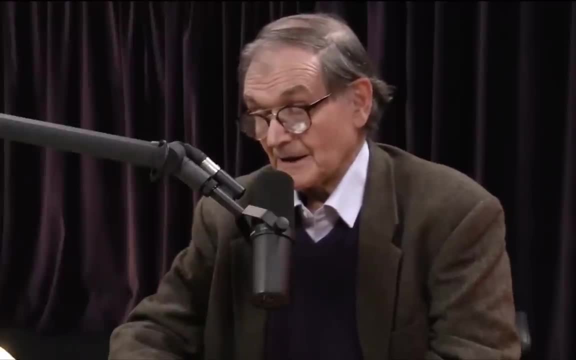 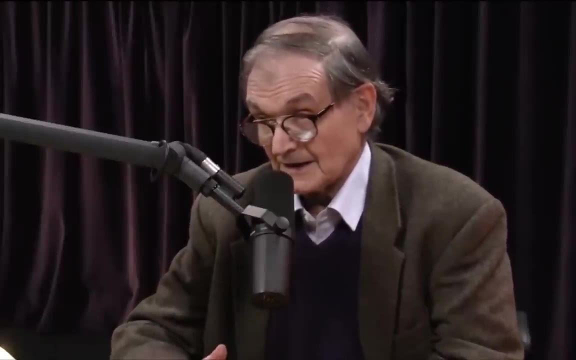 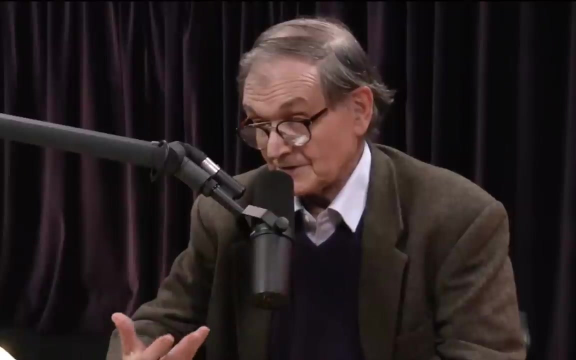 Now, this was amazing to me, because it tells me that, okay, you cannot formalize your understanding in a scheme which you could put on a computer. You see, this statement which Gödel comes up with is something you can see on the basis of the same understanding that allows you to trust the rules. 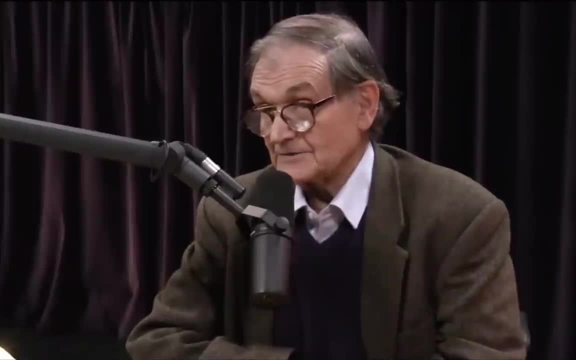 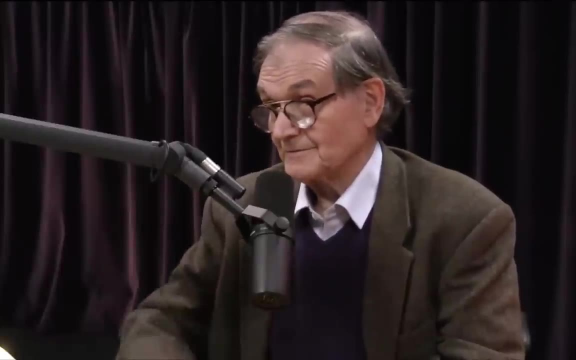 that it's true, But that it's not actually derivable by the rules. You see, it's true by virtue of your belief in the rules, And this, to me, was amazing.